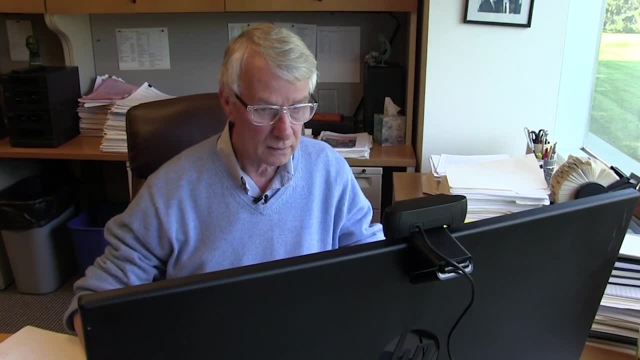 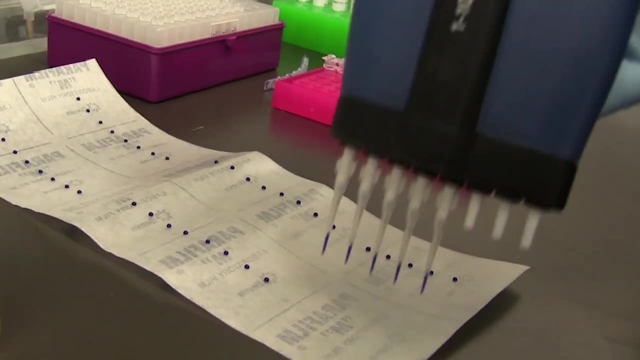 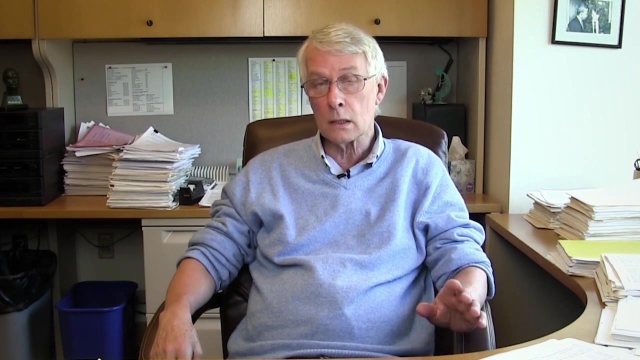 and another. We just never know. So until we have had a good chance to look at the extent of the diversity and especially to sequence the diversity that is out there, we're not going to know, And unfortunately, what is happening is that the diversity is disappearing at an enormous rate. 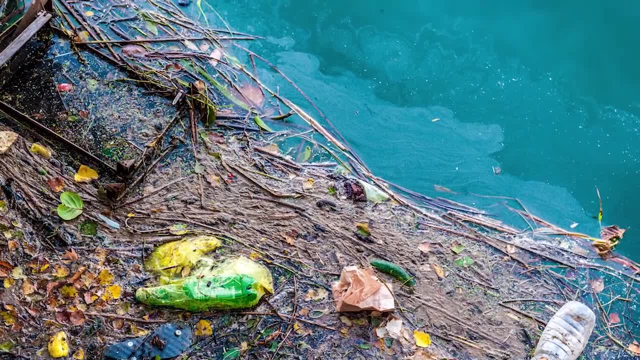 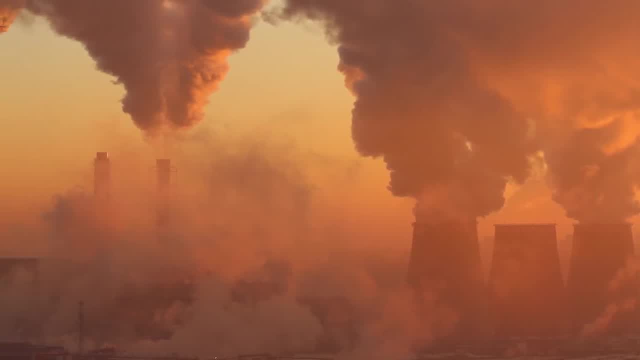 Species are disappearing. We're polluting the environment. We're polluting the environment- Everything that we find, including the atmosphere, which is causing global warming. We're polluting the seas, which are now filling up with plastic that we throw out The landfills around the earth. 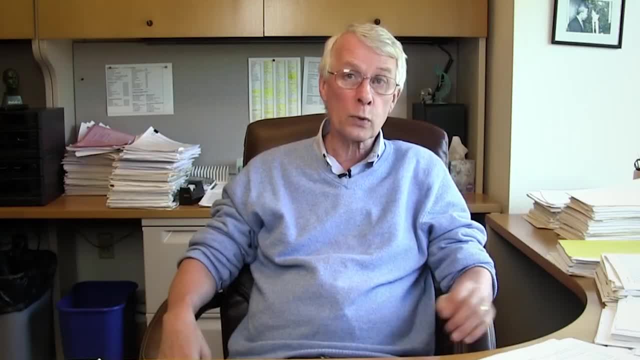 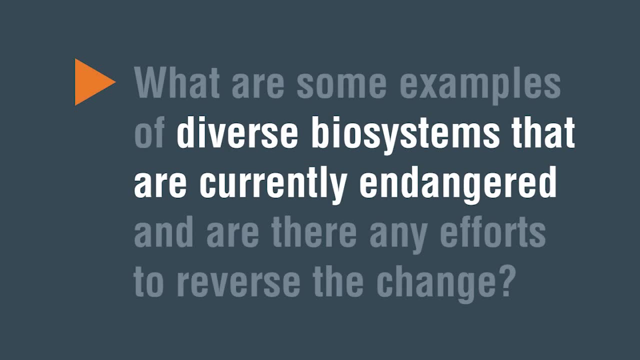 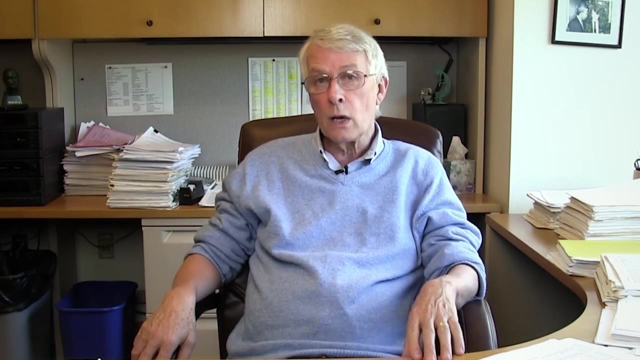 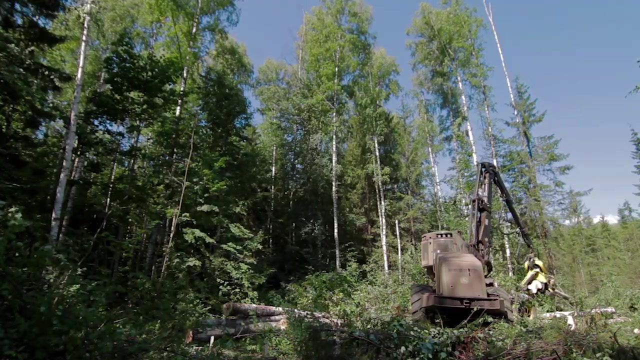 are filling up with debris And they're causing a lot of problems and they cause species to die out, Right, So you know, among the biodiversity that we have there's a lot of diversity, And we know about the rainforests- certainly in the Amazon are under constant threat because farmers 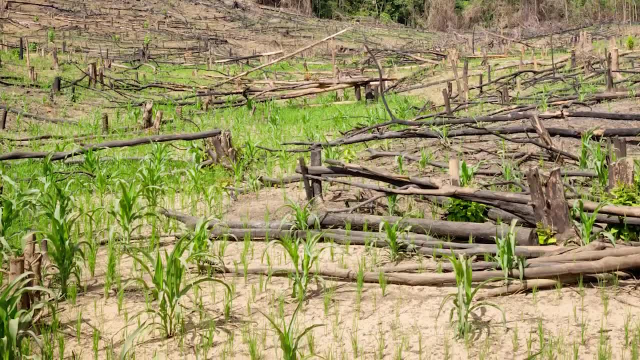 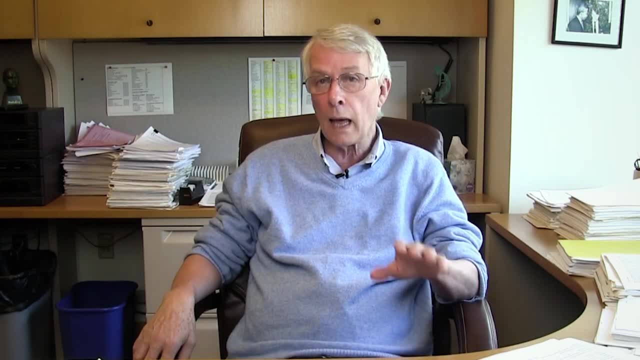 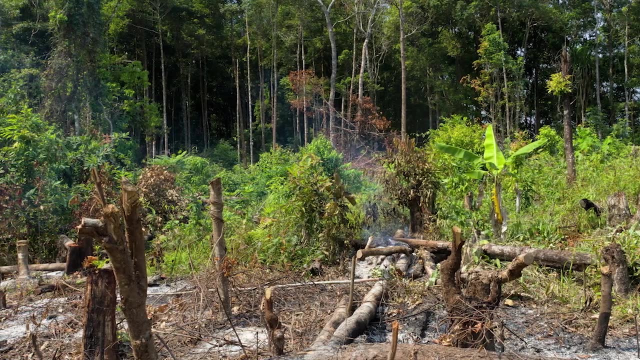 are out there taking down the trees. They're trying to use the land to grow crops, usually to not very good extent, because the land itself is usually not very good for growing crops. But nevertheless, people- farmers- are going down there. They're destroying the Amazon rainforest. 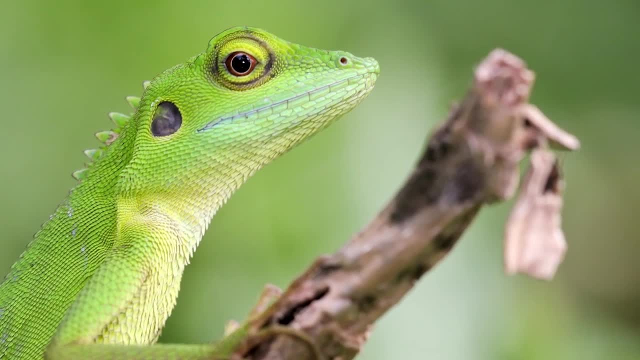 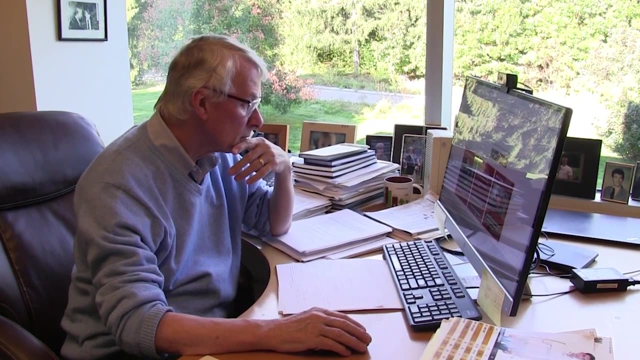 And so the natural diversity down there, which is about as extreme as anywhere you go on this planet that we know about, is just disappearing rapidly. The same is happening in Borneo, in the rainforests in Borneo, where we have the Malaysians. 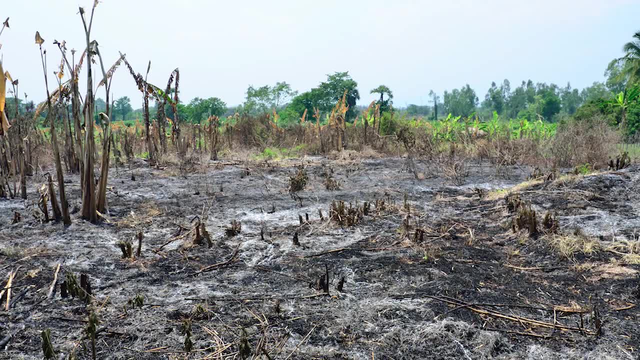 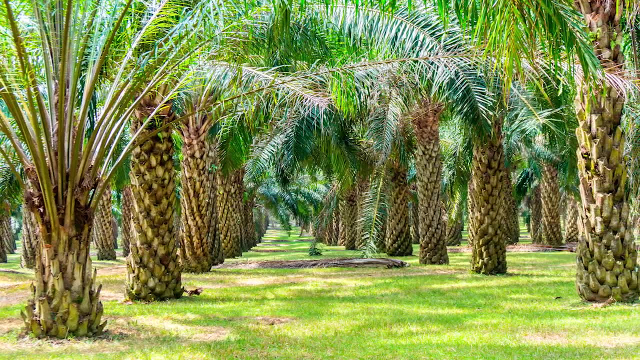 and the Indonesians, who are busy cutting down the trees there in order to grow crops that they want to grow- palm oil being the principal example of what's going on over there- And in the process they're destroying the habitat of animals like orangutans. 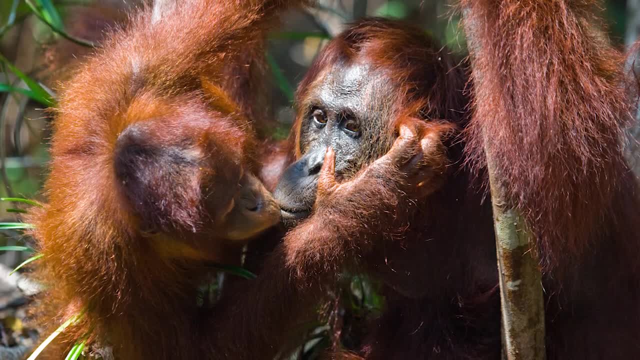 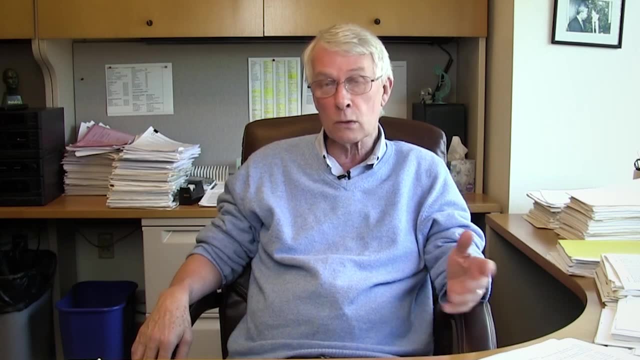 And I don't know if you've ever seen an orangutan in person, so to speak, but they're the most adorable animals you could wish for, And the last thing we should be doing is reducing their ability to live by taking down the habitat in which they hang out all day. 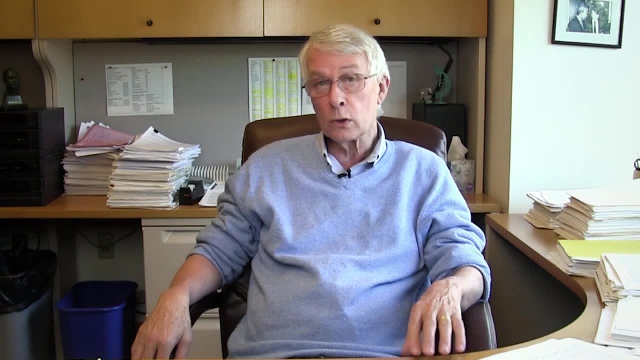 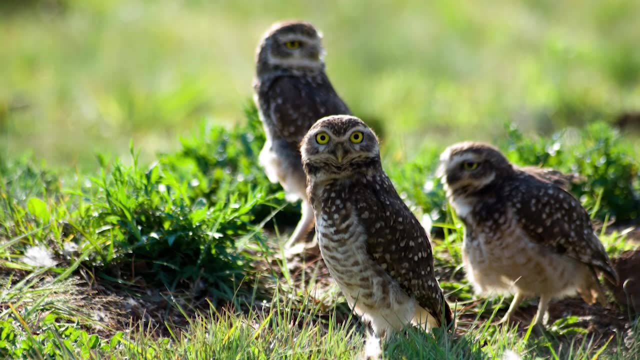 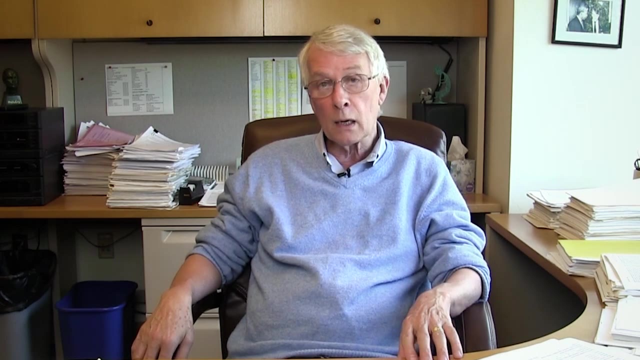 Well, I think the first thing that an individual can do is to become aware of it. So I think education, education is very important, so that people are aware that there is this biodiversity all around us. They should be aware of how useful it is. And once they become aware of it and realize that it is, 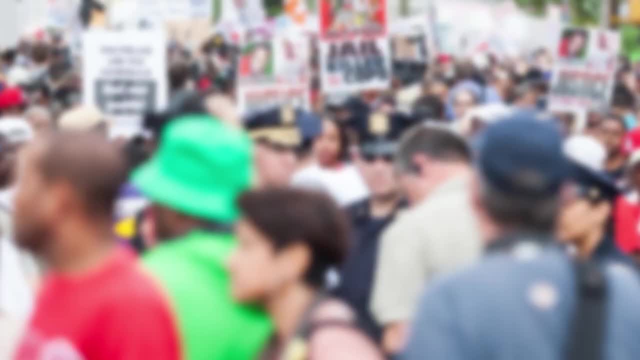 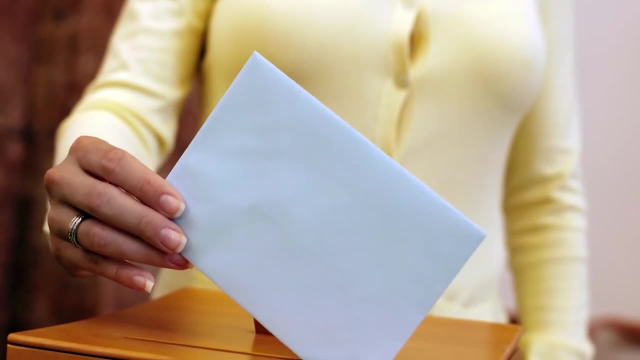 actually very valuable, then this is the time when they can start to take action, And so one of the actions they can take is to become politically active, to make sure they vote for politicians who support the preservation of biodiversity, and also to donate. 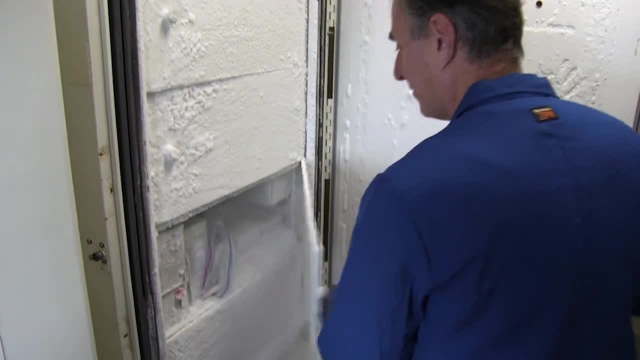 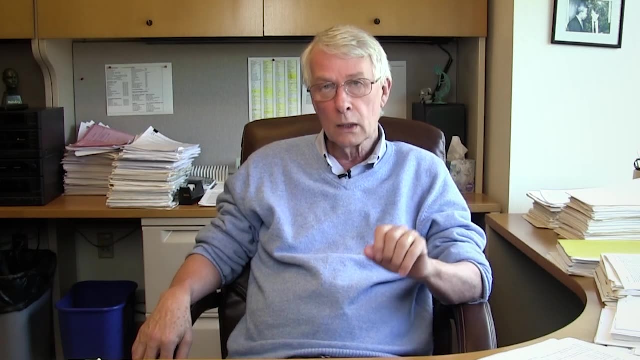 And I think that's important, because if you don't do that, then you're not really going to have the same effect on the population, And so I think that's important. I want to go back to NGOs- non-government organizations- that are trying to protect the biodiversity. 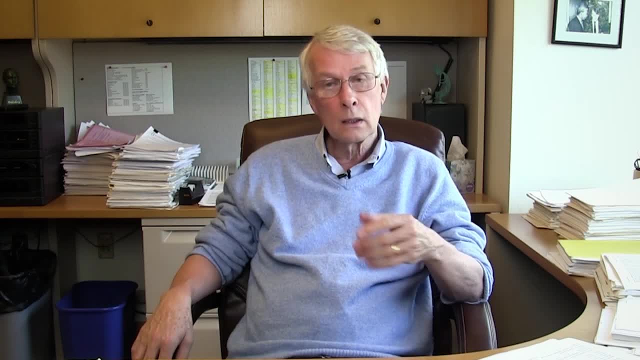 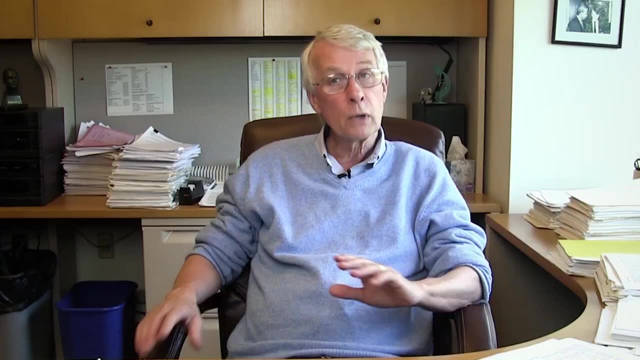 But I think it is important to make sure that, in doing so, you don't just think about biodiversity as being the be-all and end-all of everything. People have to live too, And so what you want to do is to find a nice balance between making sure that we have the land and the crops available that people need in order to eat. 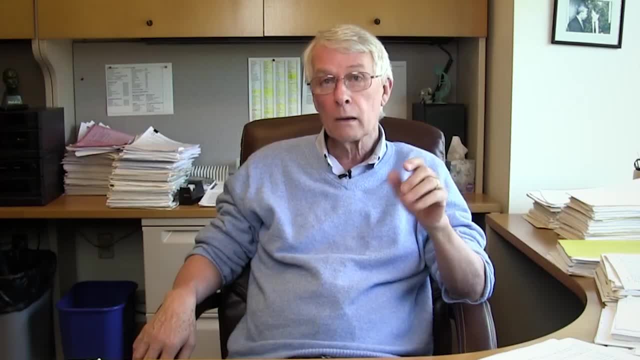 But that, at the same time, we maintain the biodiversity, And so that's an important point. Thank you very much. Thank you very much. You're welcome. Thank you very much. biodiversity as best we're able, And one of the nice things these days is that, because of 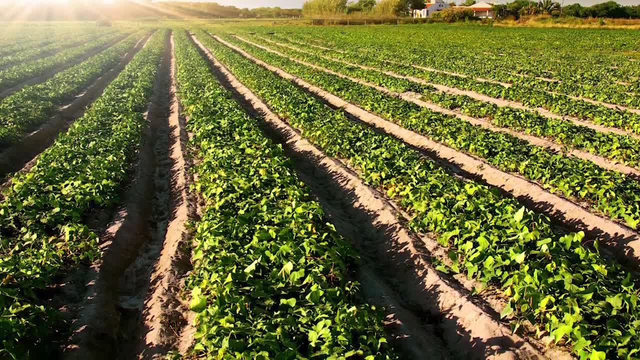 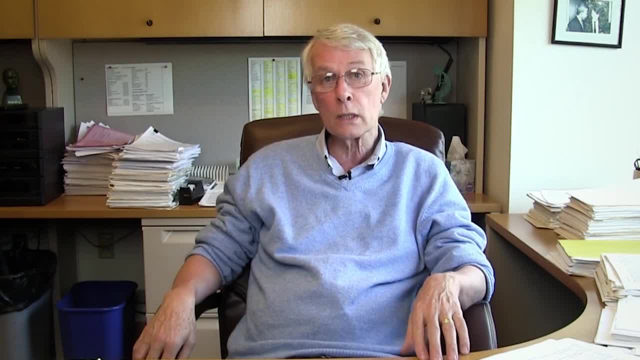 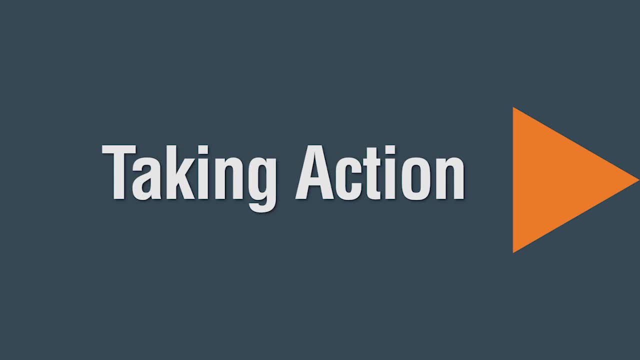 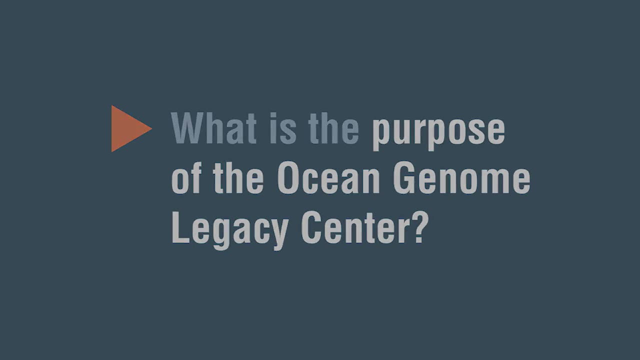 improved agricultural practices, both agronomy and the GMO movement, we can grow more food on less land than we used to, And so now we can use the excess land and use it to preserve biodiversity. So, as you know, the oceans are facing a variety of threats due to human activity. 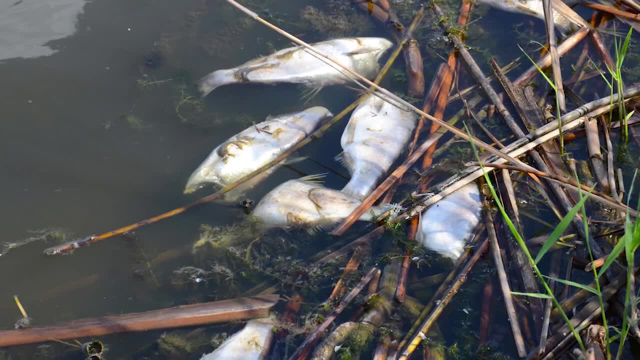 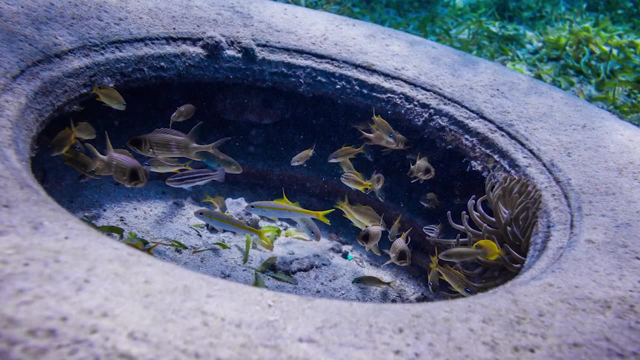 And, as a result, we're losing species from the oceans at rates we've never seen before. As we lose those species, we're not only losing these incredible animals, but we're also losing the information in their genomes. That information is extremely valuable. It can be. 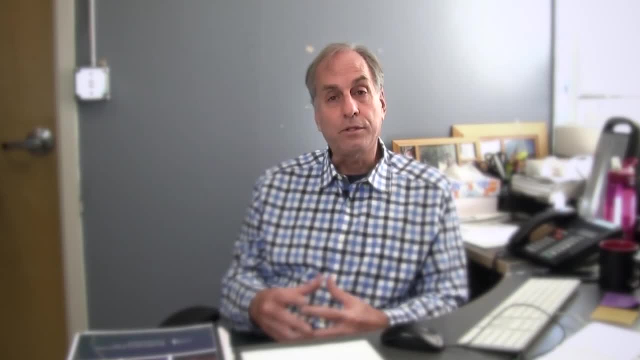 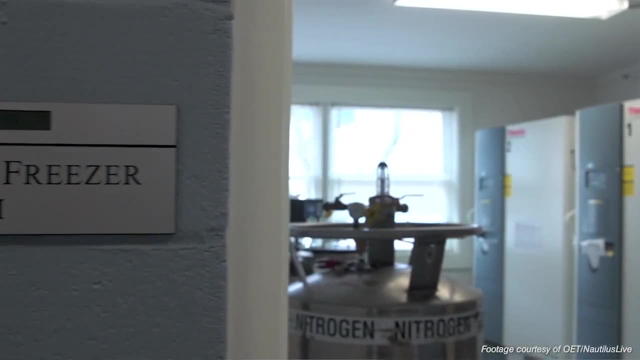 used to create new species. It can be used to create new species. It can be used to create new species, It can be used for medicine, for biotechnology, And so, to try to prevent the loss of that information, we've created the Ocean Genome Legacy Collection. Basically, it's a bank. 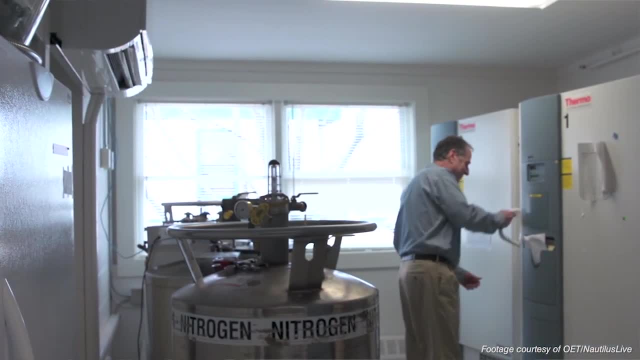 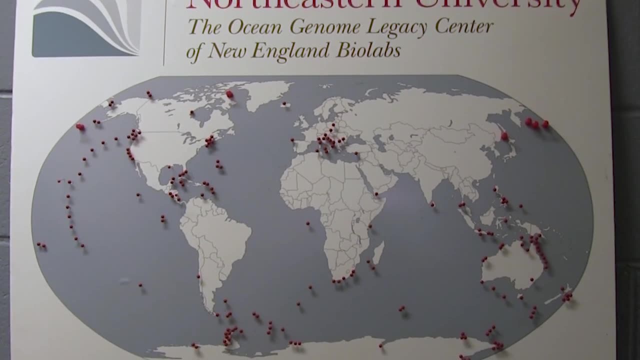 or a library of DNA samples and tissue samples from a whole variety of different marine organisms collected all around the world. And what's most important about that collection is that we make that collection available to the scientific community to support research that can help us protect the oceans. 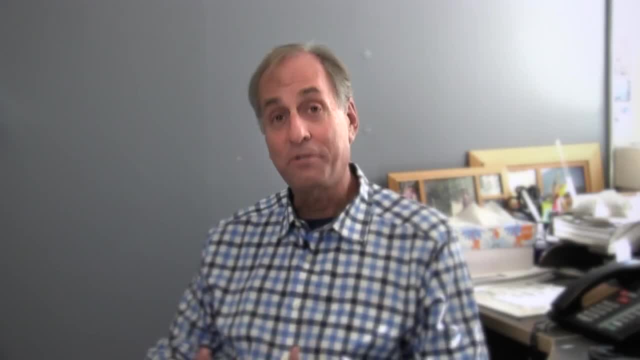 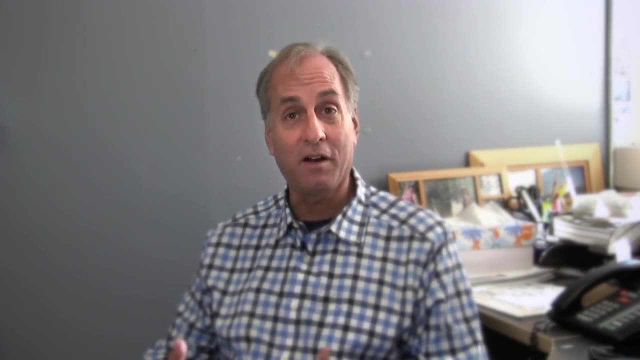 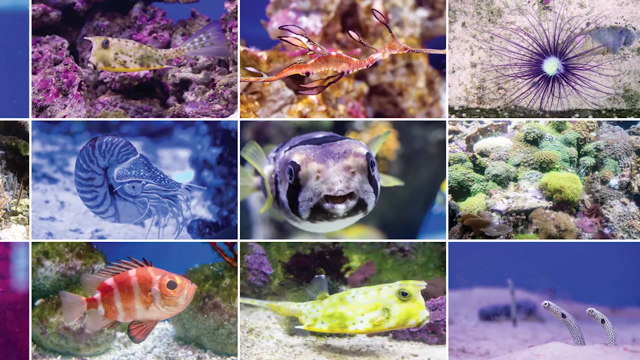 So it's extremely important to study the biological diversity of the oceans, because it really represents the lion's share of diversity on our planet. For example, scientists divide the animal world up into 31 major categories. We call them phyla. It turns out that of the 31 phyla, 30 have 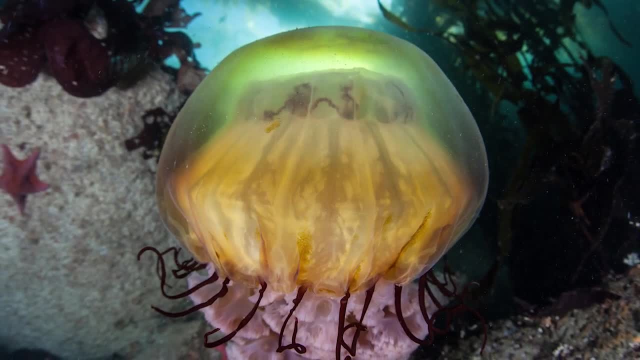 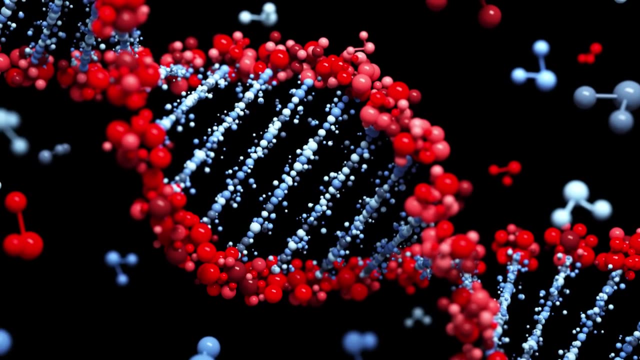 representatives that are found in the ocean. So there's only one phylum that has no marine representatives. So for that reason we're not going to be able to do a lot of research on the ocean. We really have to look at the ocean if we want to understand the deep biological diversity of life on our planet. 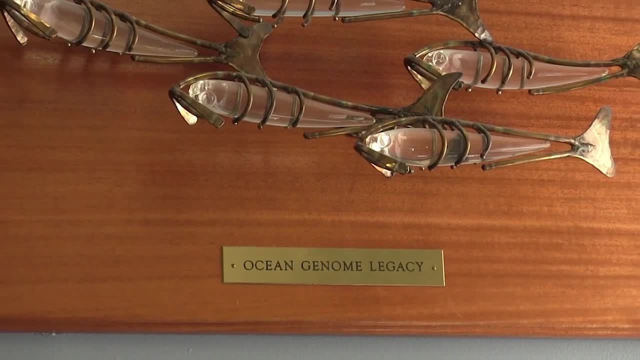 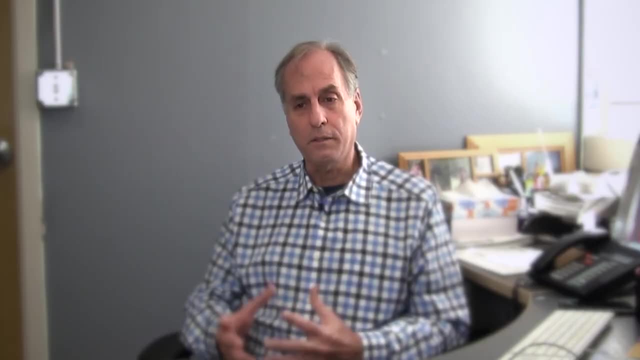 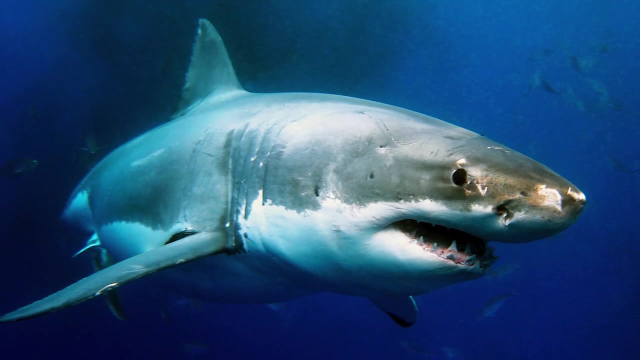 So actually the Ocean Genome Legacy was sort of the brainchild of Don Combe, the founder of New England Biolabs. Back in the year 2000, Don read an article, an opinion piece, that appeared in Science and it asked the question: why aren't we saving DNA from the world's threatened and endangered species? He 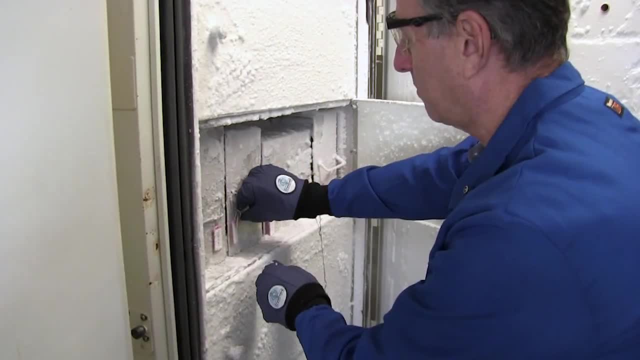 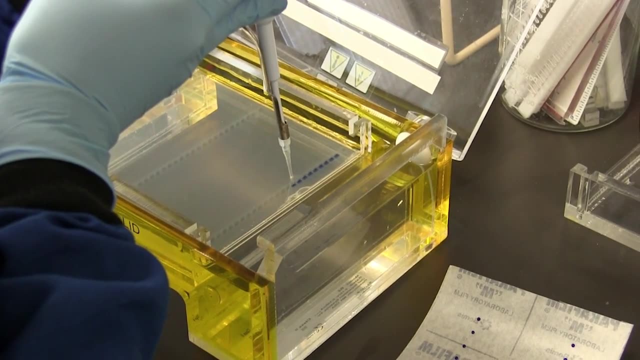 realized that it doesn't have to be. It's not just the DNA that's threatened and endangered species, It's the sense of being stronger and stronger. It's the way of thinking. So Don realized that we shouldn't just take any new technology, that we had everything we needed to do, that It just took someone to take the. 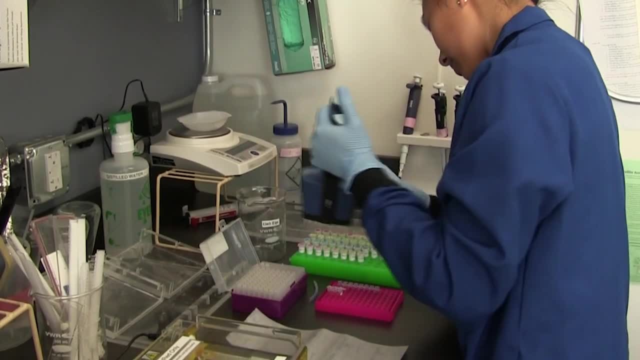 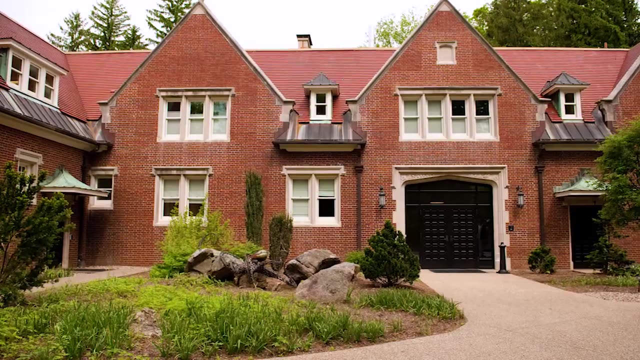 initiative And Don realized that he could do something about it, So he founded the original board of the Ocean Genome Legacy From there we spent about 10 years at New England Biolabs figuring out how to create the Ocean Genome Legacy Center, what we should do and what we should become, And at some point we recognized that. 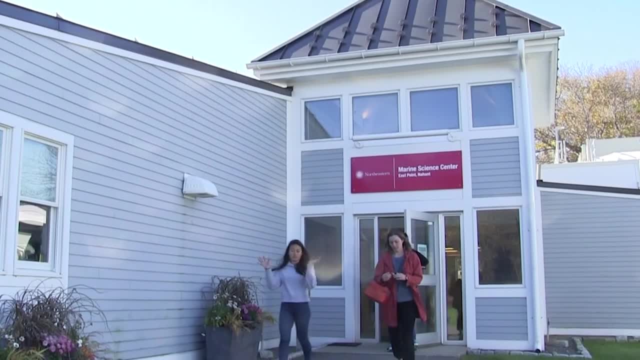 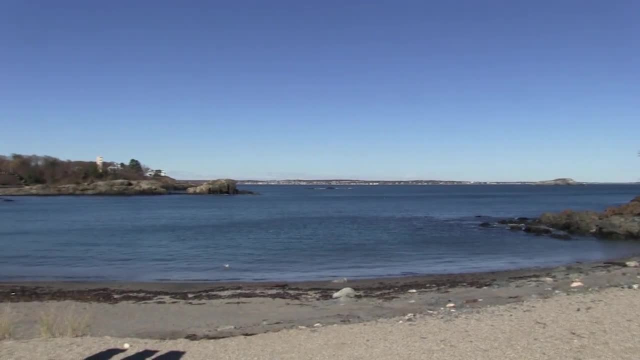 it would be a great advantage for us to be associated with a new technology and a new way of developing our, for us to be associated with a major research university like Northeastern University and also a marine science center that is located right on the coast, and so we made the move here to 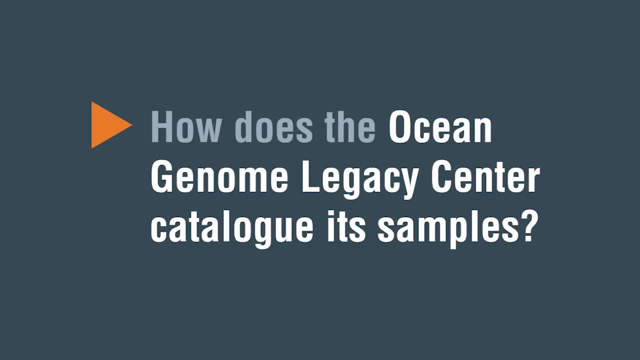 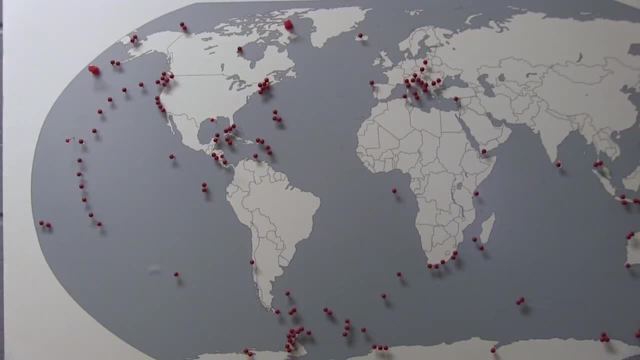 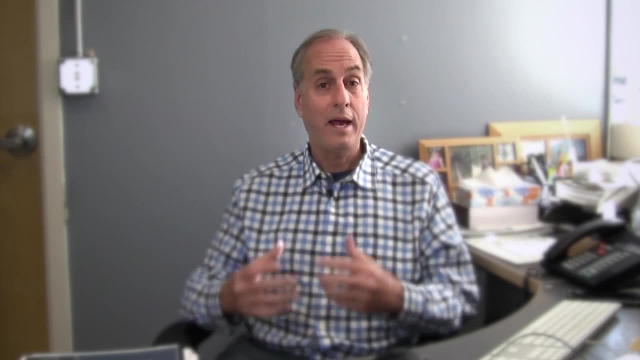 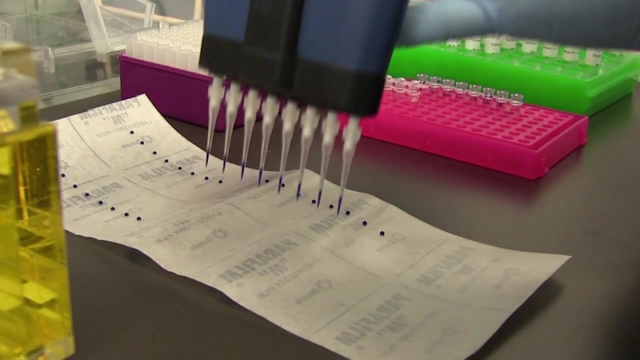 Northeastern University. So typically we receive samples from scientists all around the world. These can be tissue samples or DNA samples, or sometimes even whole organisms. When we get them we have to document the correct species names for them. We take photographs, We do a variety of things to clean them up.